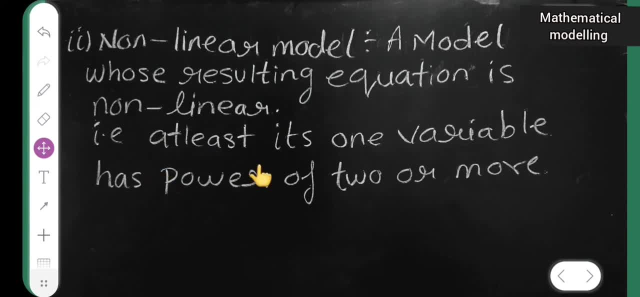 resulting equation is non-linear, that is, at least it's one variable- has power of 2 or more. Okay, let us see the example of what is a non-linear model. It's a very simple definition. a model whose resulting equation is non-linear is called okay, that is, at least it's one variable. 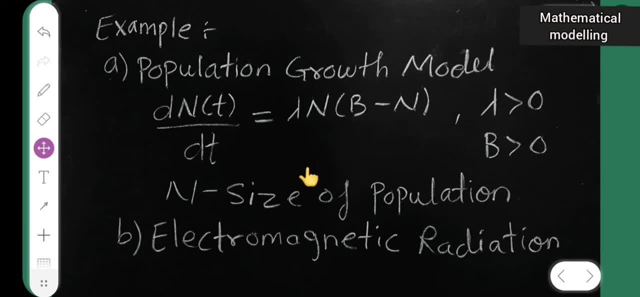 has power of 2 or more. What it means is example population growth model. So I have taken an example of the population growth model. Again, I am differentiating with respect to t, this n of t, that n is the size of the population, which is equal to lambda, is the decay constant, and n of 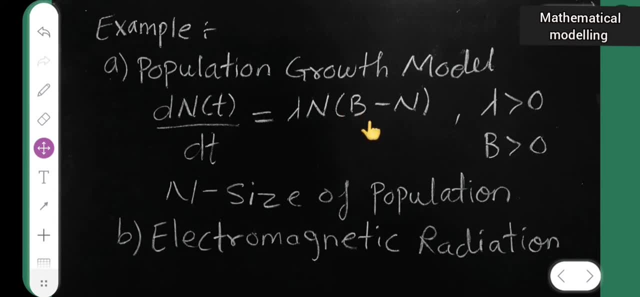 b minus n. This is what birth and death, Birth minus death. Okay, your lambda is greater than 0 and birth is also greater than 0.. Okay, because b is positive, birth is positive and n is negative. the death rate is negative, So it is less Okay. so if you. 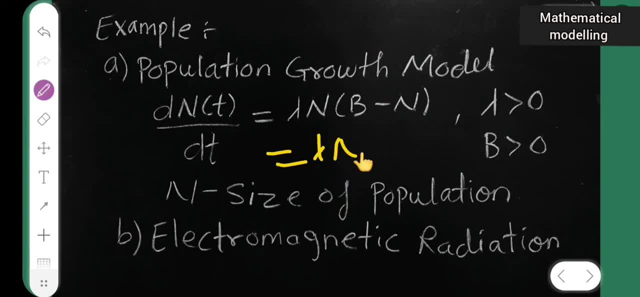 all do it like this: lambda n b minus lambda n square. So what I have said is what I have said is: lambda n b minus lambda n square. So what I have said is what I have said is: pop, it's one variable, has power 2 or more. Okay, at least it's one variable. See here, it is the. 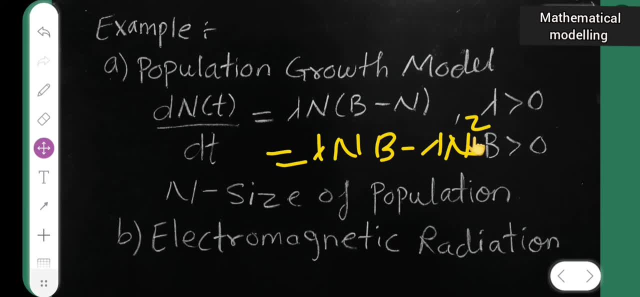 power is 1, but at least one variable has power 2 or more, So it has power 2.. So this is the example of a non-linear model. Okay, so if you substitute this properly, if you do it properly like this, minus this into this, okay, Okay, then next is what electromagnetic radiation is? one more example. 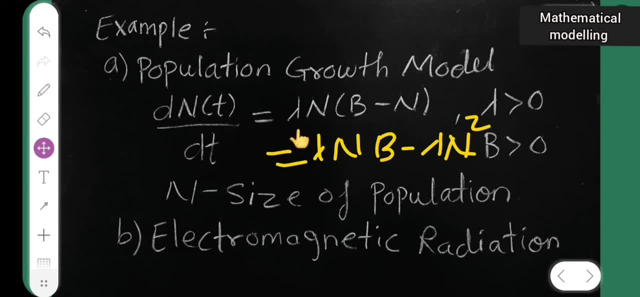 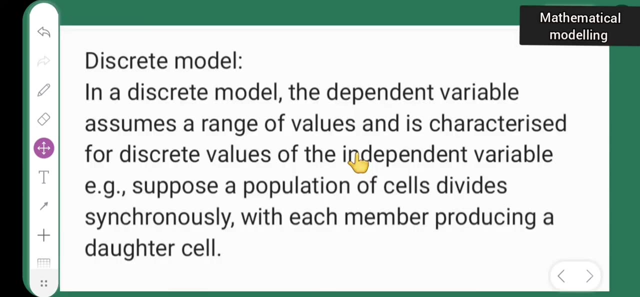 of the non-linear model. Here we are not substituting anything, You just have to solve it: lambda n b minus lambda n square. So this square is what it is. what power? 2. So it is non-linear model. Okay, I hope you all have understood this. Next is the district model. Now let us see what. 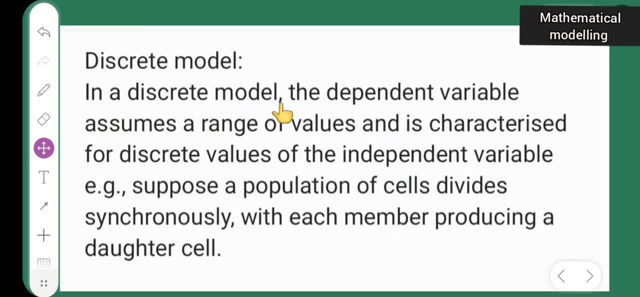 is a district model. In a district model, the dependent variable assumes a range of values and is characterized for district values. of the dependent variable Example is here. suppose a population of a cell divides synchronously with, synchronously with each member producing a cell. Okay, then there is one more example of a district model: Annual plant produces seeds at 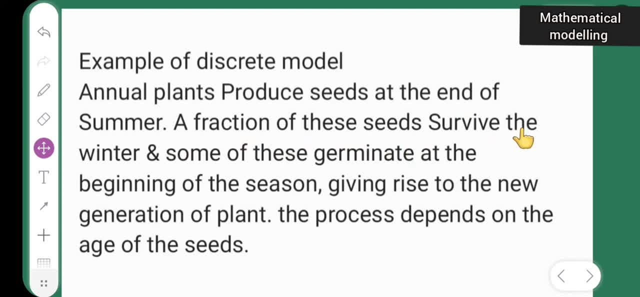 the end of the summer. A fraction of this seed survive the winter and some of this germinate at the beginning of the season, Because rise to the new germination of plant process depends on the age of the seeds. Okay, so basically what happens over here? it lies between somewhere in the interval. 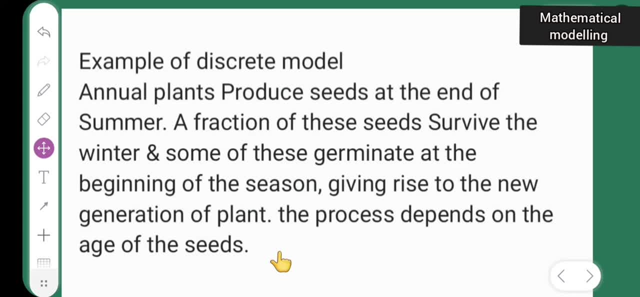 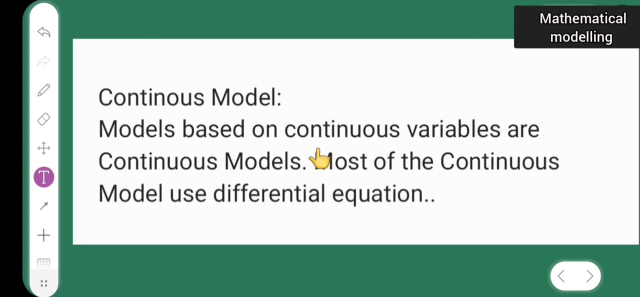 because in the summer what happens? the leaves start falling down and in winter it start. In winter, it will give rise to the new generation of plants, Okay so. so, basically, it lies between the an interval. Okay, next is continuous model. Let us see what is a continuous model now. Okay, so, continuous model. 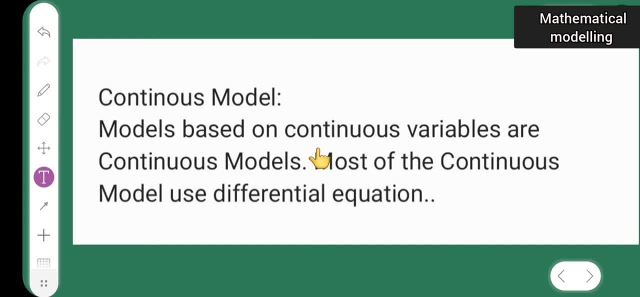 model based on continuous variable model. Wait Okay, model based on continuous variable are continuous models. Most of the continuous model use differential equation. Okay so, like PD, OD, like that way. Okay so in a continuous model it depend on variable. assume in a continuous model, dependent variables. Okay so. 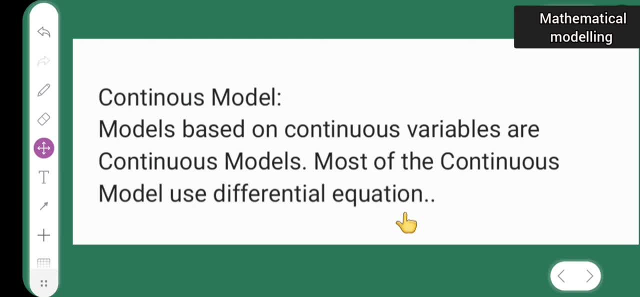 basically, this is the way it works. Now you can see. let me explain you all this thing. In a continuous model, dependent variable assume continuous. Most of the continuous model results in a differential equation like OD or PD, The derivative being constant. Rates of change. continuous model are similar only when analytic solution are available. okay, So 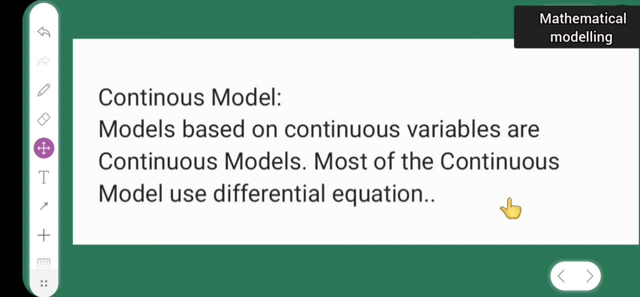 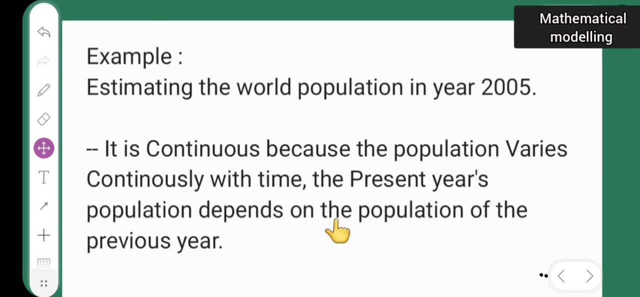 basically, this definition is very easier than whatever I said just now. So you can see that. Okay, that is all. So we will end the topic here, Bye, Bye, Bye, Bye. this definition only. Next is the example of the continuous model. First is the estimating: 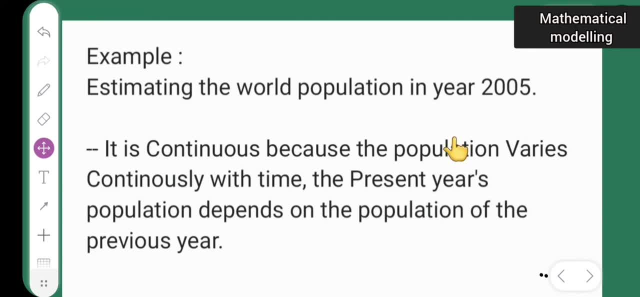 the world population in year 2005.. It is continuous because the population varies continuously with time. The present year is what the present year population depends on the population of the previous year. So here what happens is happens. it is continuous because the population 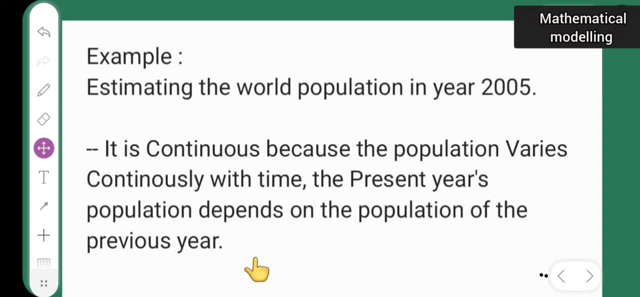 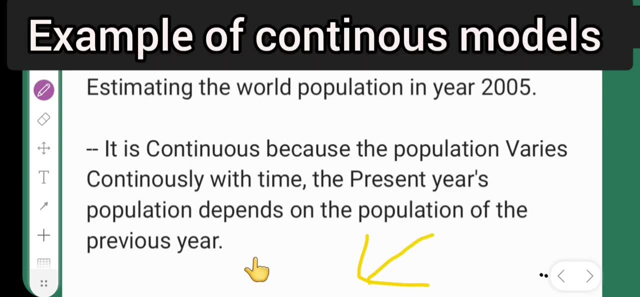 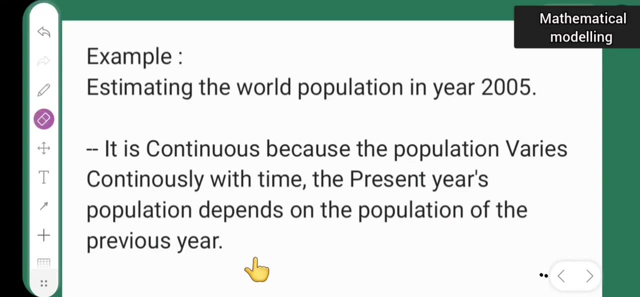 varies continuously with time. The present year population. it depends on what? yeah, the present year population depends on the previous year, So it will be continuously. it will be moving. So, yeah, okay, next let us see what it is. Next is the static order, So 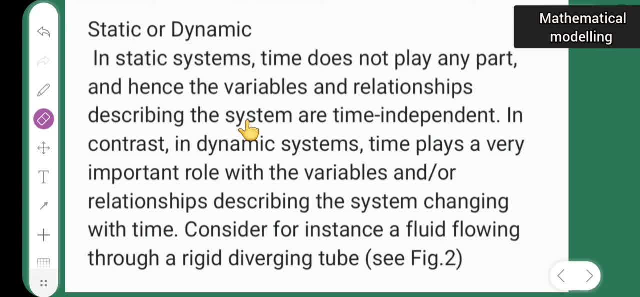 dynamic model. So let us see what is the first one, that is, the static model. Time does not play any part. Okay, time does not play any part and hence the variables and relationship describing the system are time independent. In contrast, in dynamic system, time placed. 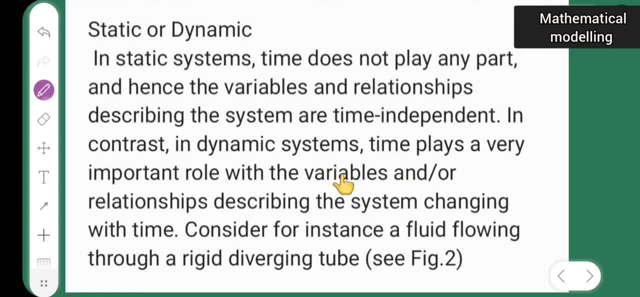 in the dynamic system, So in dynamic system. time placed in the dynamic system, So in, whereas when we, if we talk about, this, is a static system where time does not play any part, and here comes the dynamic part, okay here. So what is the dynamic here? So here. 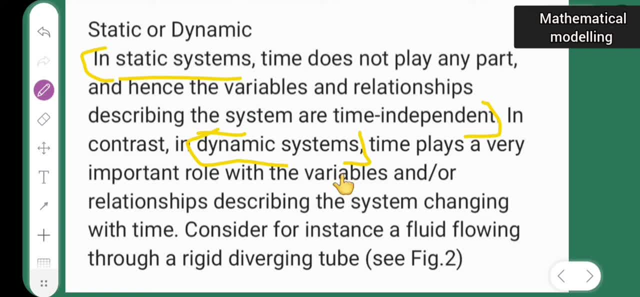 from here to here. this is the definition of the static. okay, No need for this, So directly start studying from here. So in dynamic system, time plays a very important role, with the variable and or relationship describing the system changing with time. So now what? 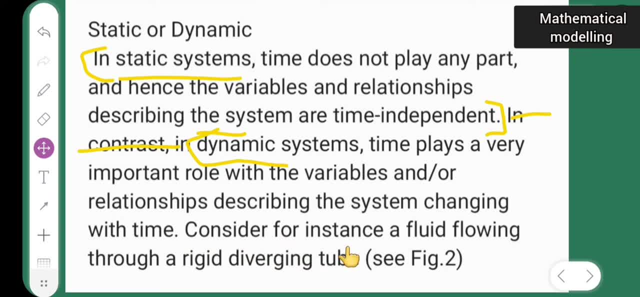 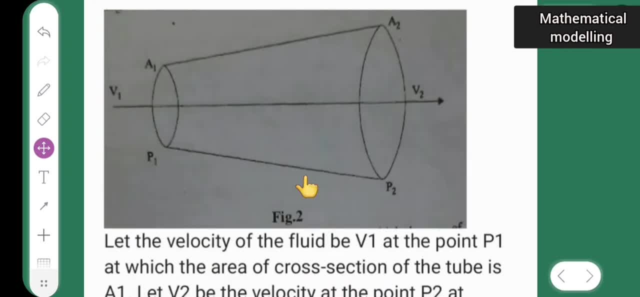 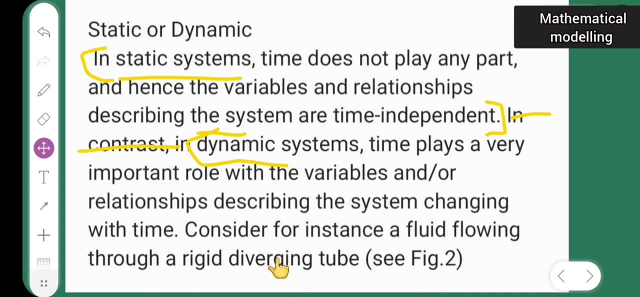 I have been doing is I will be considering. consider, for instance, of fluid flowing through a rigid diverging tube. okay, So this is the fluid, This is the fluid. So this is the figure 2, where we are considering the fluid flowing, the rigid diverging tube. 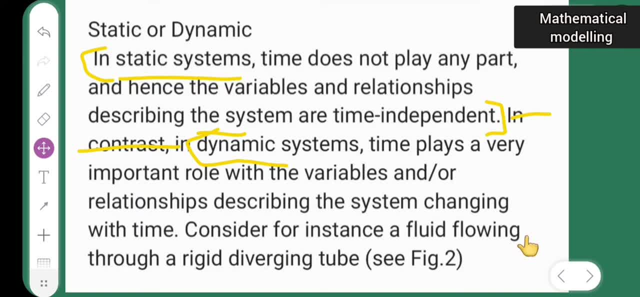 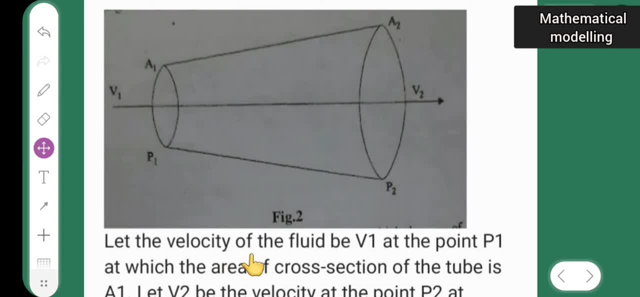 So this is the rigid diverging tube where the fluid is flowing towards to that, okay. So let the velocity of the fluid v1- this is the v1- let the velocity of the fluid v1 at the point P1: okay. At the point P1 at the point P1 at the point P1: okay. At the point P 1: okay, So I am figuring. 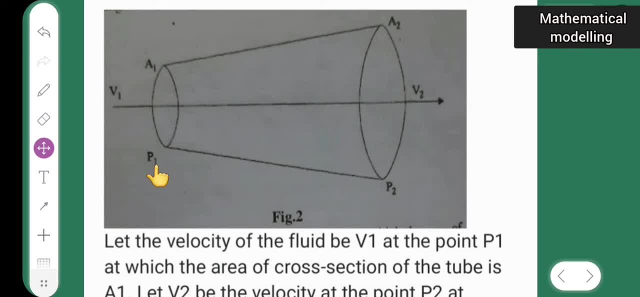 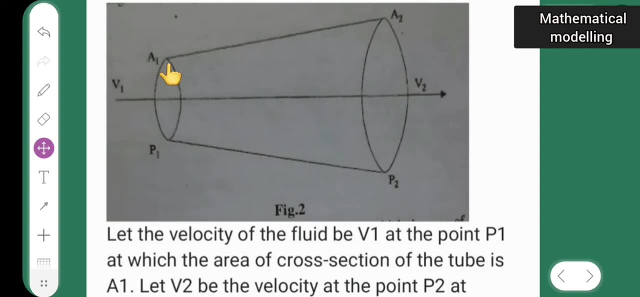 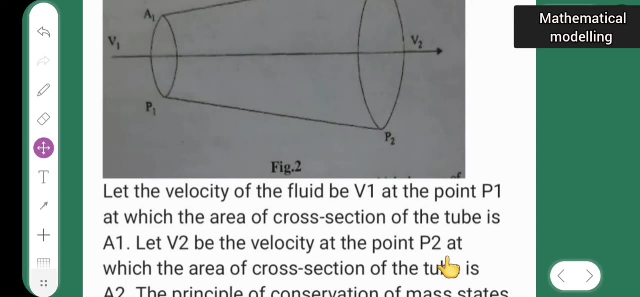 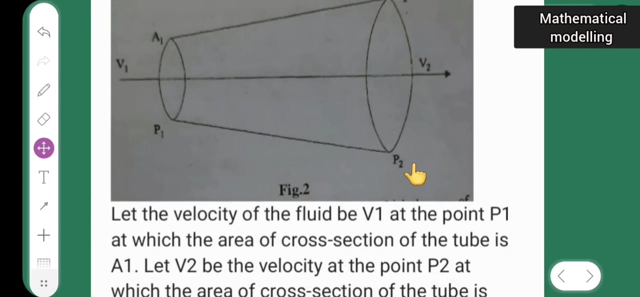 point P1, at which the area of cross section of the tube is A1. okay, the cross section of the area of the tube is what? A1? okay, now next is what? let V2 be the velocity at the point P2. okay, so V2 be the velocity at point P2, at which the area of cross section of the tube is. 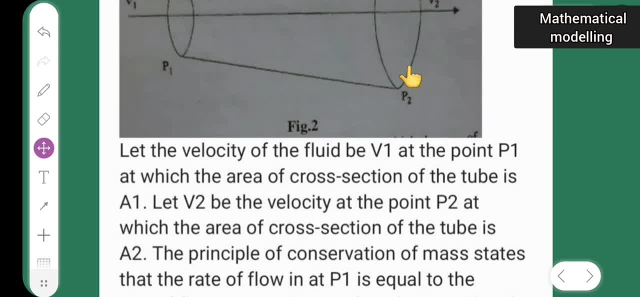 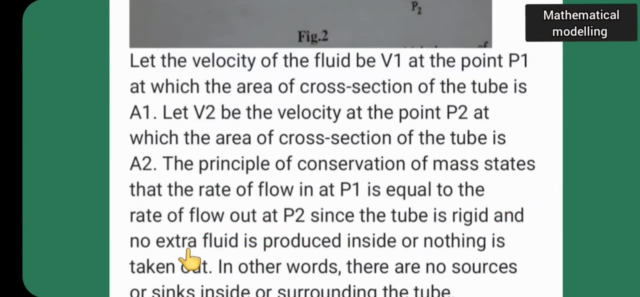 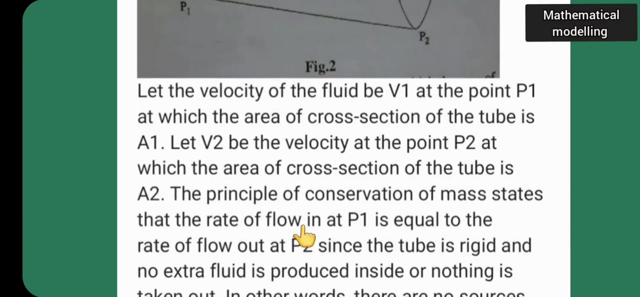 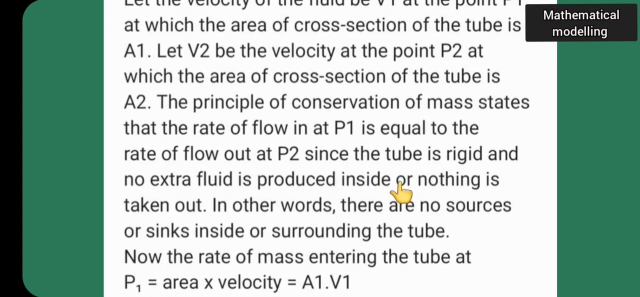 A2. okay, the principle of conversation of mass states that the rate of flow in at P1 is equal to is equal to what rate of flow out at P2? so flow will be out at P2. okay, over here. this next is what? Since the tube is rigid and no extra fluid is produced inside or nothing is taken out, 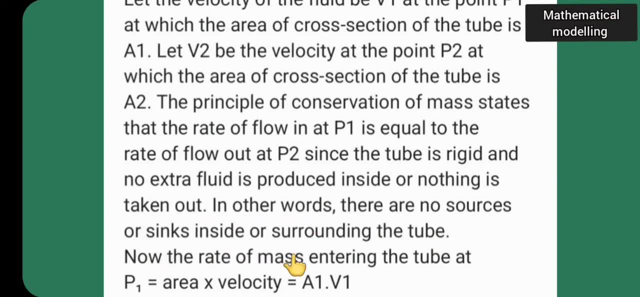 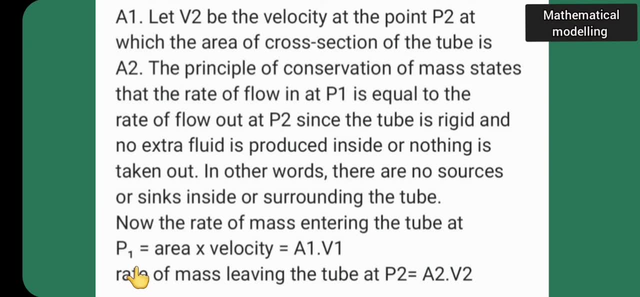 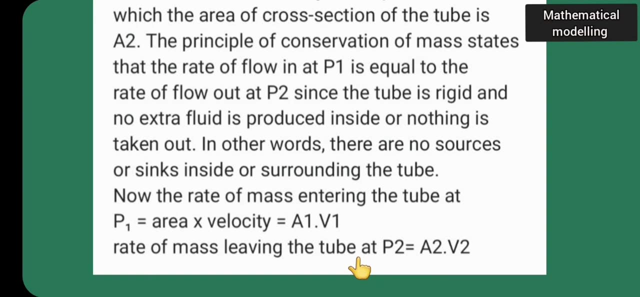 in other words, there are no sources of sink inside or surrounding the tube. now, the rate of mass entering the tube at P1 is equal to area. into velocity, which is equal to area, is what. A1 into velocity, V1 and rate of mass of leaving the tube is what. 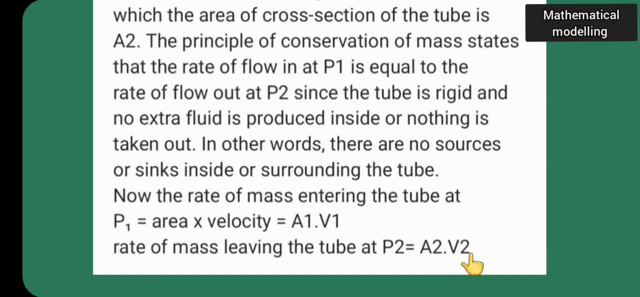 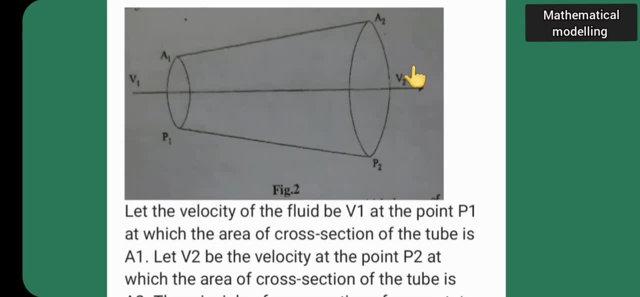 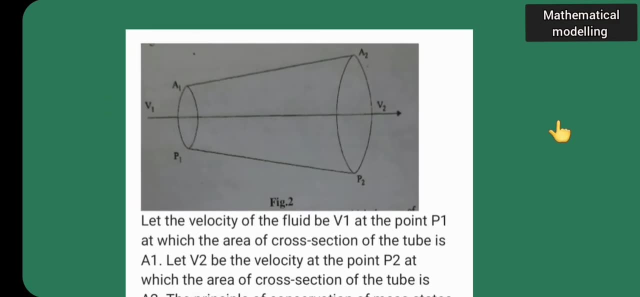 Area into velocity, like this is A2 into V2. this is where the rate of mass is leaving the tube. so this is the where it is leaving the tube. okay, here it is entering and here it is leaving the tube. okay. so you all can see the diagram over here. you all can copy. 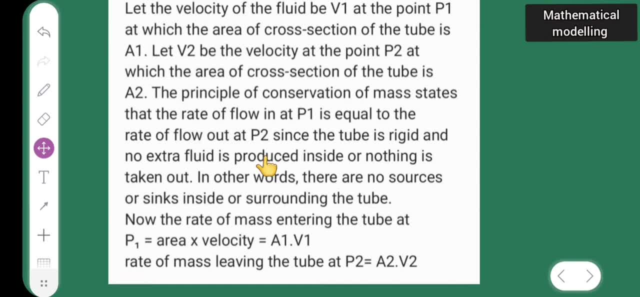 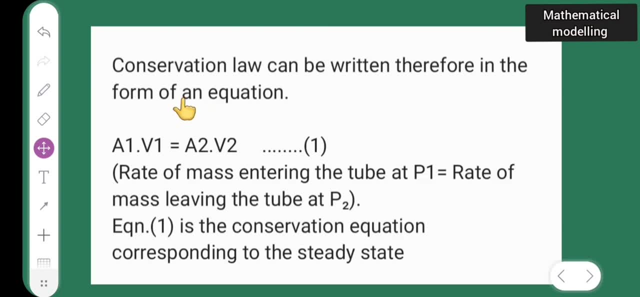 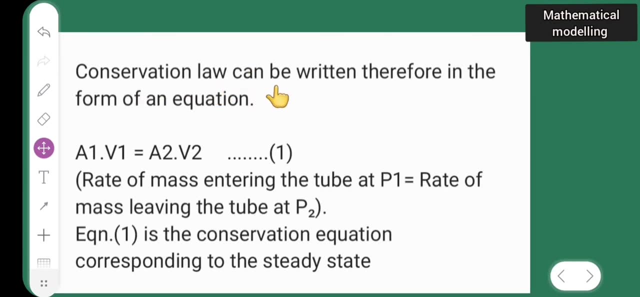 down the example of that and here is the from here you all can copy down this thing. okay, let me. Okay. So here comes the conversation of conversation. law can be written, therefore, in the form of the equation that is: A1 into V1 is equal to A2 into V2. okay, this is where the, where 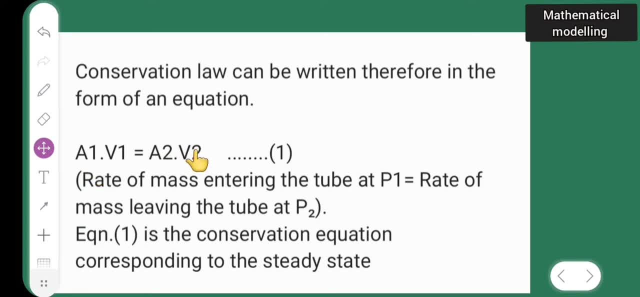 it is entering the tube and here where it is leaving the tube. okay, and take it as one equation. one Rate of mass entering the tube at P1 is equal to area into velocity, which is equal to area of mass leaving the tube at P1 is equal to rate of mass leaving the tube at P2. okay, 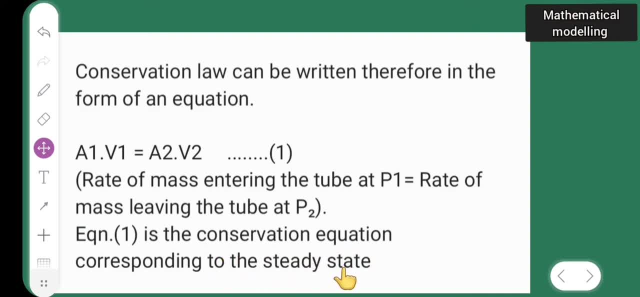 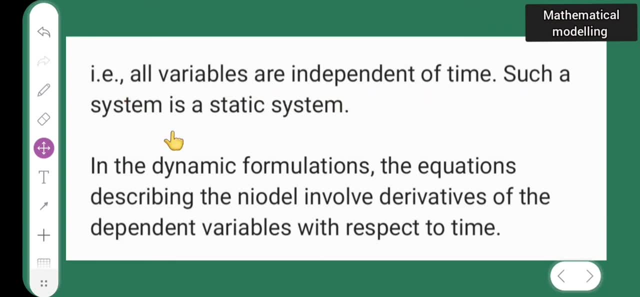 Now, equation one is a conversation equation corresponding to the steady state. next, that is, all variables are independent of time. such a system is a static system, okay, so, whereas all variables are independent of time, right, so such a system is called what? static system? so this is an example of a static system, okay. 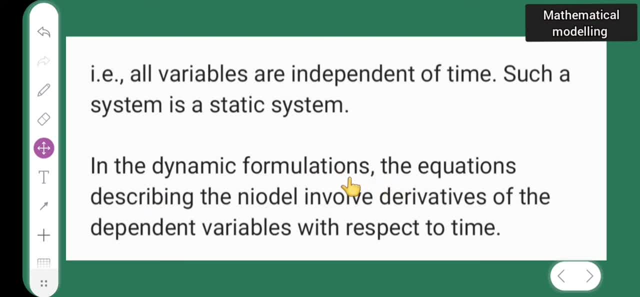 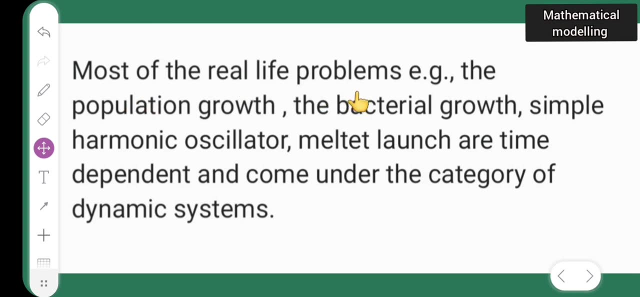 Okay, Now comes the dynamic formulation, the equation describing the nodal involved derivative of the independent variable with respect to the time Now. most of the real life problems- example: the population growth, the bacterial growth, simple harmonic oscillator, magnet launch- are time dependent. so these are all time dependent. 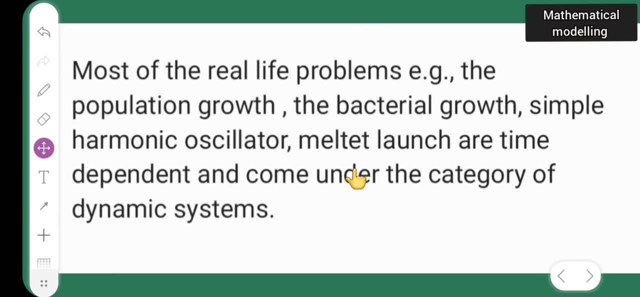 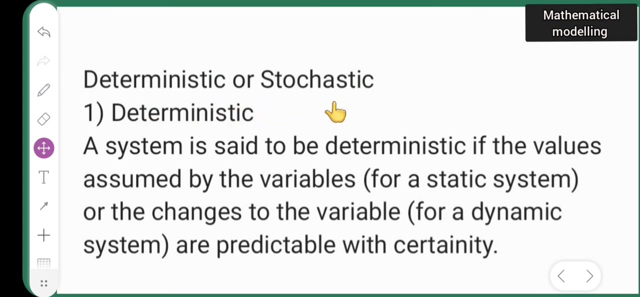 and come under the category of dynamic formulation. Okay, So these are all the examples of the dynamic system. so this is the example of what dynamic system. so this is an example of dynamic model. okay. so next let us see what is deterministic or stochastic. okay, so first is the deterministic. what is the deterministic? a system is said. 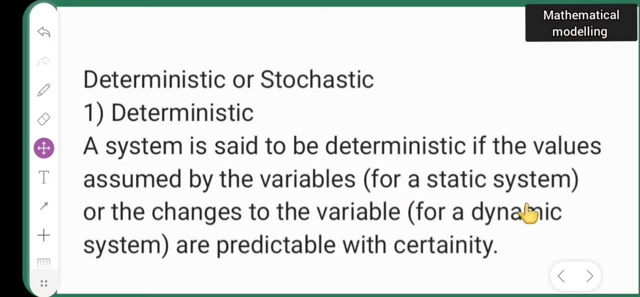 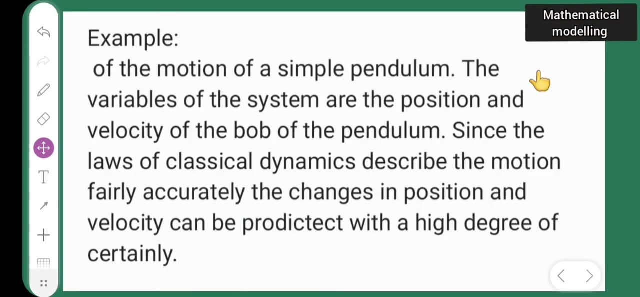 to be deterministic if the values assumed by the variables for a static system in the bracket right now, or changes to the variable for a dynamic system are predictable with certainty. only if the values assumed by the variables or changes to the variable are predictable with certainty. okay, it is called deterministic. now what are the example of that? if it is? 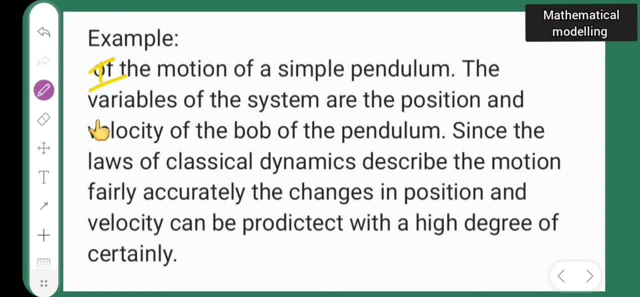 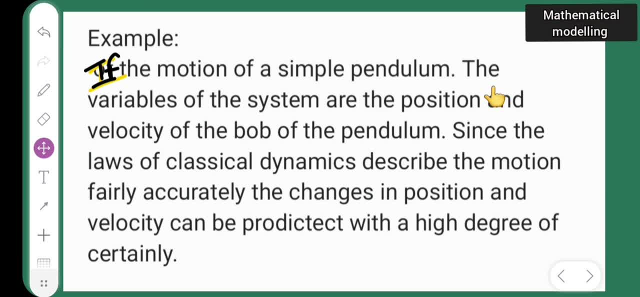 Okay, let me see that quickly. okay, if the motion of simple pendulum, the variables of the system are the position and velocity of the bob of the pendulum, Okay, Okay, okay, since the laws of classic, since the law of classical dynamic, describe the motion. 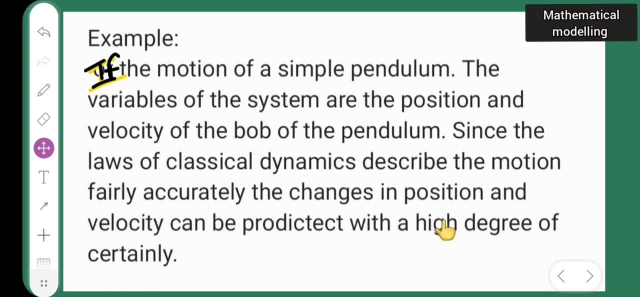 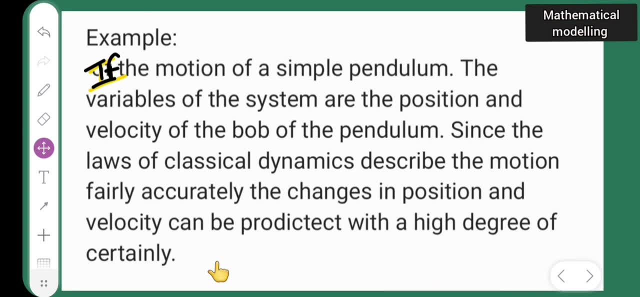 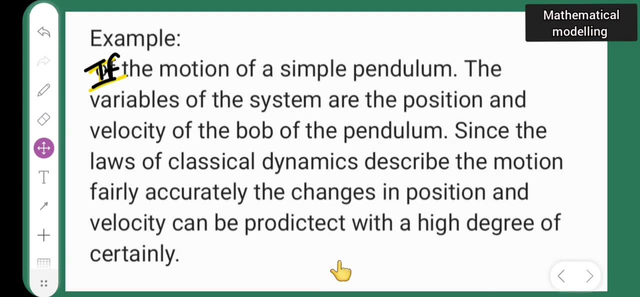 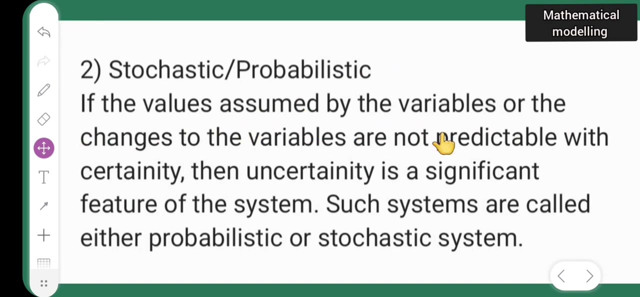 fairly accurately. the changes in position and velocity can be predicted with a high degree of certainty. okay, so this is an example of the deterministic model. next, let us see what is the stochastic probabilistic this thing. if the values assumed by the variables or changes to the variables are not predictable with certainty, then uncertainty is a significant 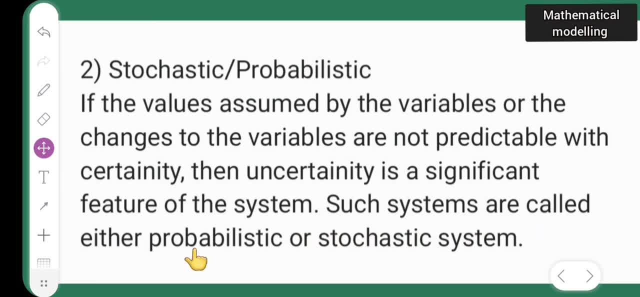 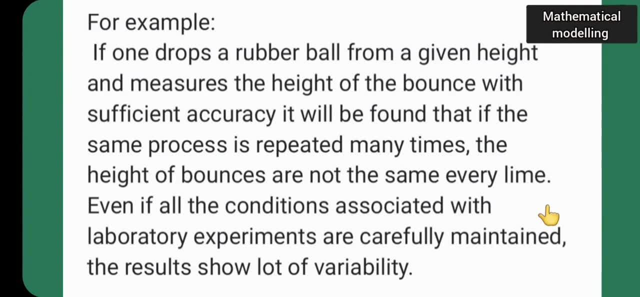 feature of the system. such a system are called either probabilistic or stochastic system. okay, so this is the definition of a stochastic or probabilistic. now let us see the example of stochastic or probabilistic this thing. if one drops a rubber ball from a given height and measures the height of the bounce with, 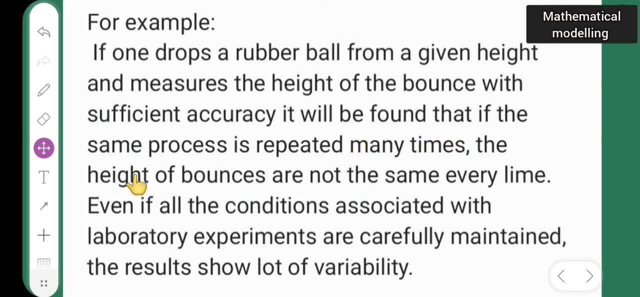 sufficient accuracy, it will be found that if the same process is repeated many times, the height of bounce are not the same every time. okay, then, even if all the conditions associated with laboratory experiments are maintained, the results show a lot of variability. so this is an example of what